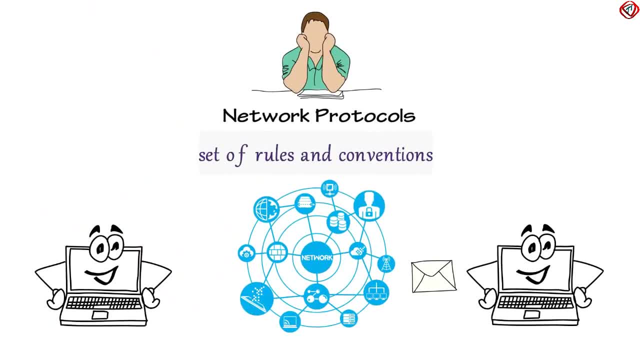 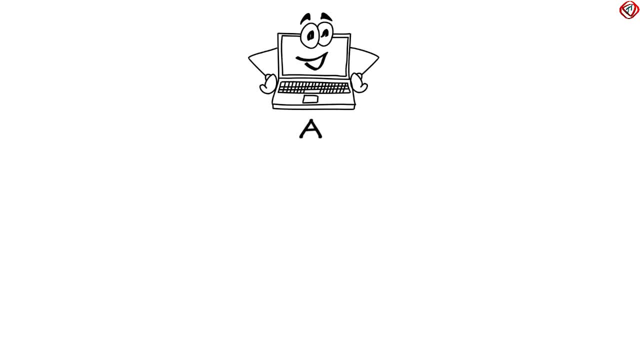 so that we can understand each other. Same is the case with computers. To transfer a file effectively, computers should follow some set of rules and conventions. Consider: computer A is transferring a movie to computer B. Consider two cases: First, when they are not following a set of rules and conventions, and the second one. 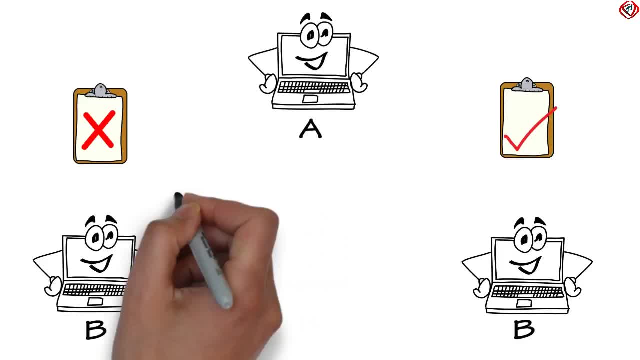 when they are following a set of rules and conventions. In the first case, computer B will pop up a message saying the file is corrupted. On the other hand, in the second case, computer B would be able to understand this file as a movie. That is, data transfer in. 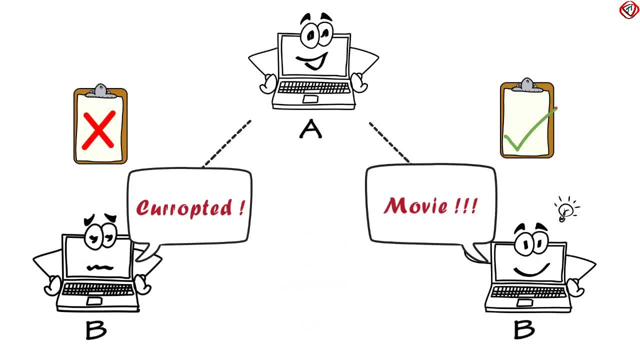 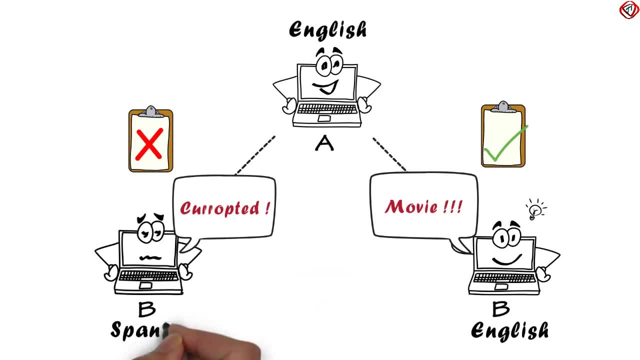 the computer B would be able to understand this file as a movie. That is, data transfer in the second case is successful because both computers followed some guidelines. It is like both computers decided to speak English, instead of one speaking English and other speaking Spanish. 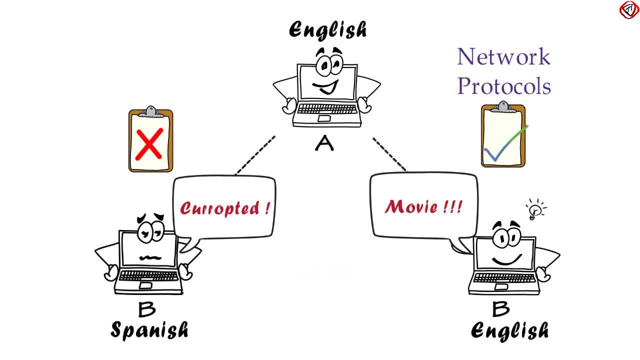 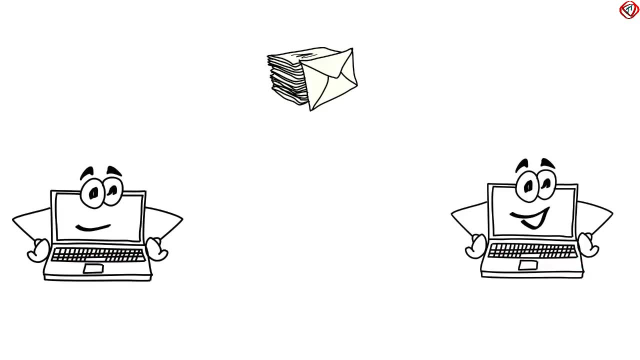 So we can say that network protocols help to make effective connections among networking devices. Modern network protocols sends data from one computer to another in the form of packets in which whole file is divided into small pieces. Some security measures are added to each packet. These packets are received and reassembled at destination to generate the original file. 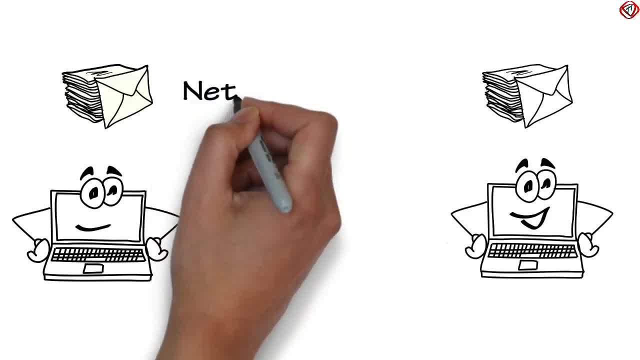 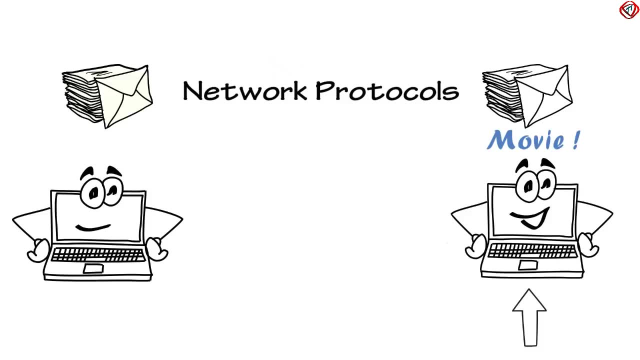 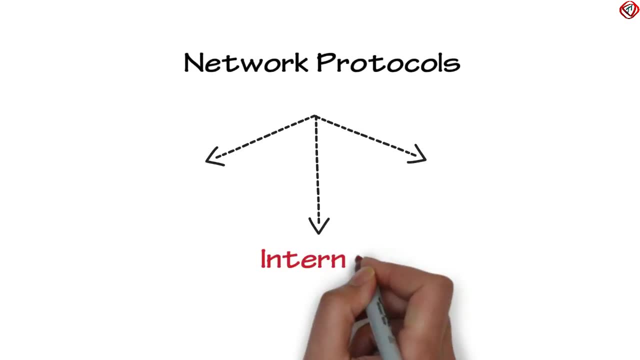 The security measures that are added to each piece are decided by network protocols, and the receiving computer will be able to understand the received packet and hence the whole file, if, and only if, it follows the same networking protocol. Network protocols include Internet protocols, Wireless Network Protocols and Network Routing Protocols. 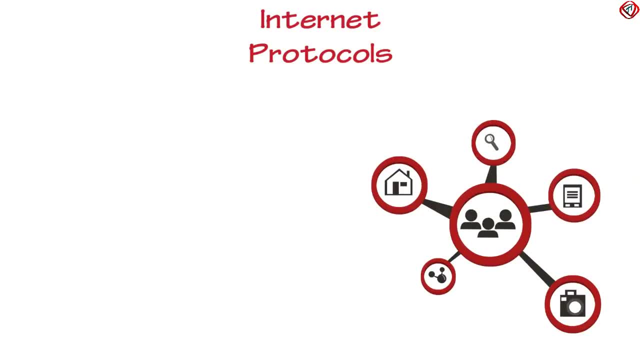 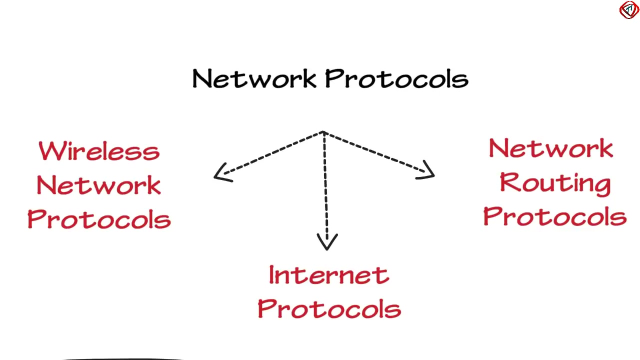 Internet protocols are needed for proper functioning of internet and includes TCP, UDP, HTTP, FTP, ARP and ICMP. These four protocols interact with applications like web browser. On the other hand, these two protocols interact with network adapters or NICs. Wireless network protocols are needed for proper functioning of Wi-Fi, Bluetooth and 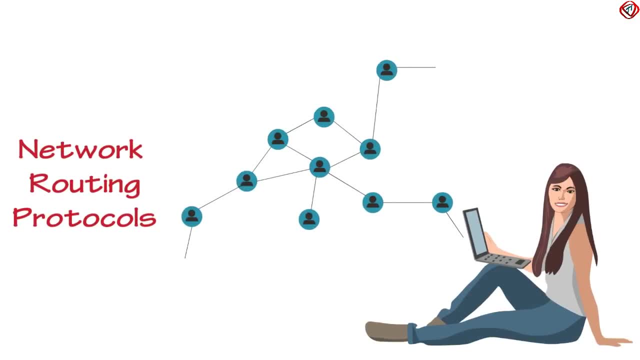 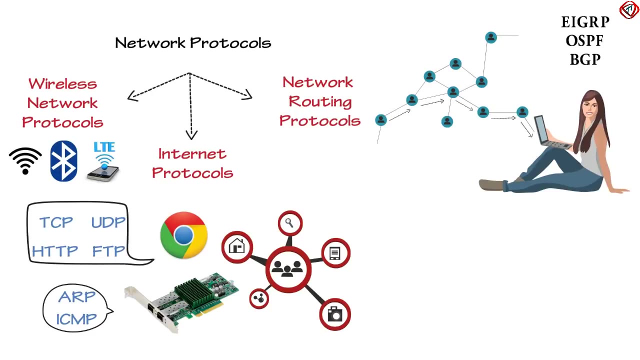 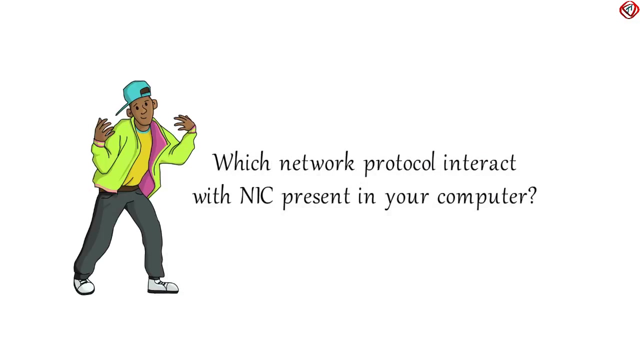 LTE. Network routing protocols are needed for deciding best download path for a device to download a file from internet. Network routing protocols include EIGRP, OS, PF and PGP. We are going to discuss these in detail in later videos. Now answer this question: which network protocol interact with NIC present in your computer?